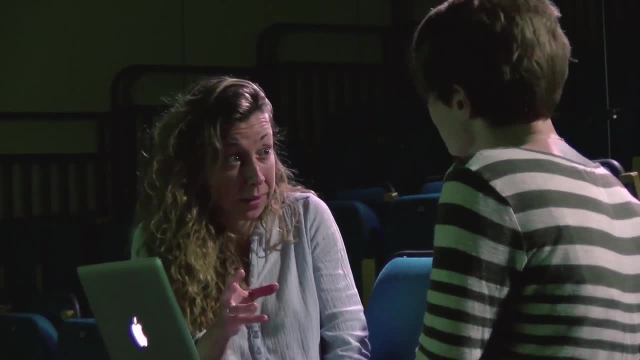 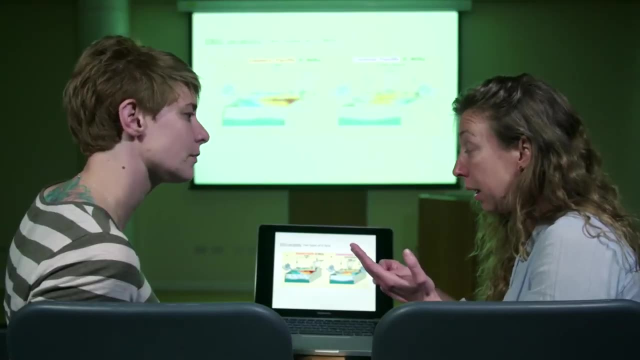 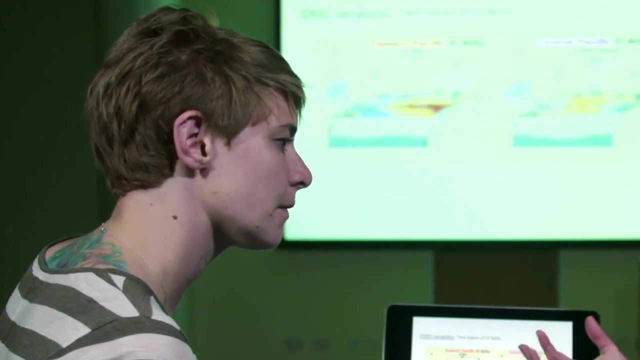 and it has a periodicity of two to seven years. So in this periodicity we encounter different types of events. Some are called El Niño, and generally they are associated with warming of the climate or of temperature, and La Niña, which might be more associated, 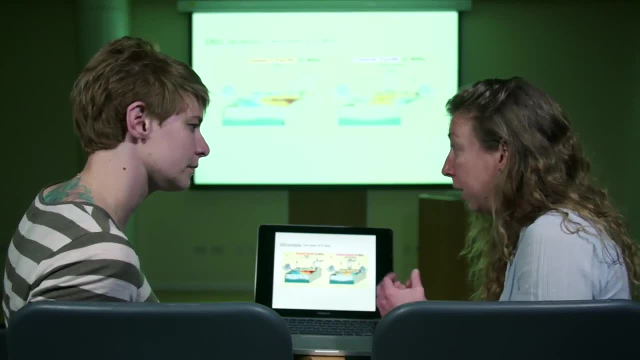 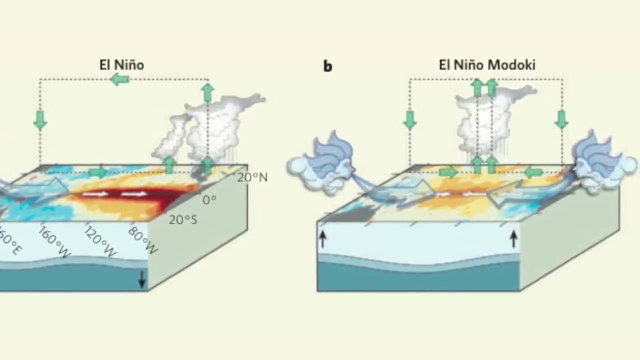 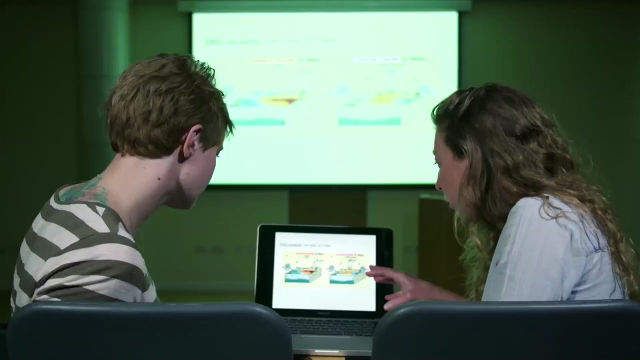 with cooling in the sea surface temperature in the tropical Pacific. So in principle we have studied the El Niño impact on the ocean biology And in fact in recent years there has been more and more evidencies that we can characterize two types of El Niño. So the characterization is based on the location of the maximum sea. 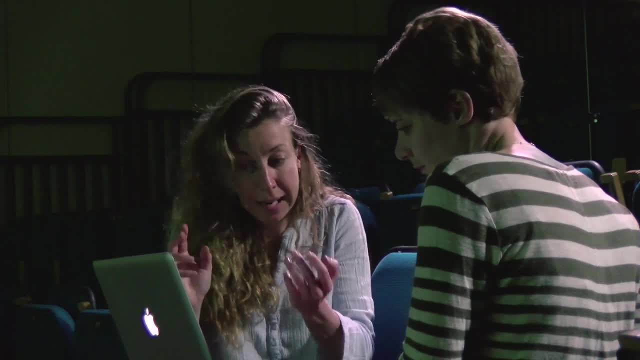 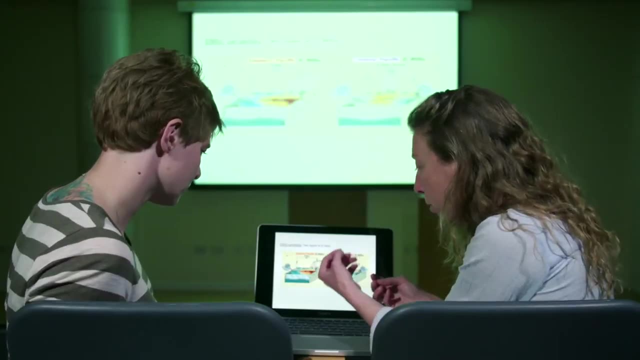 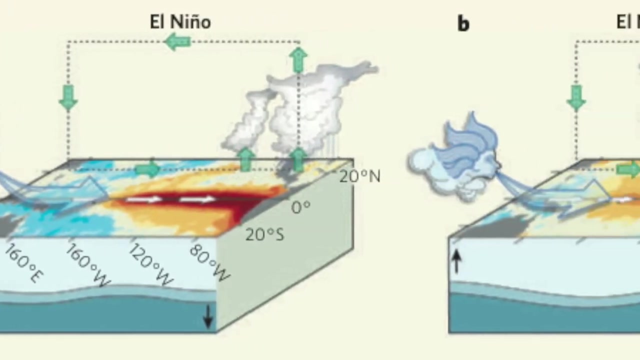 surface temperature warming. So in the more classic type of El Niño, also called as a canonical or eastern pacific El Niño, the anomalous warming of SST occur on the eastern side of the tropical pacific and, in contrast, in recent years, actually since the 1990s- there has 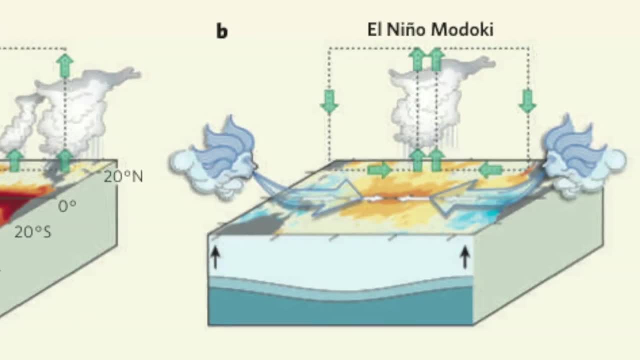 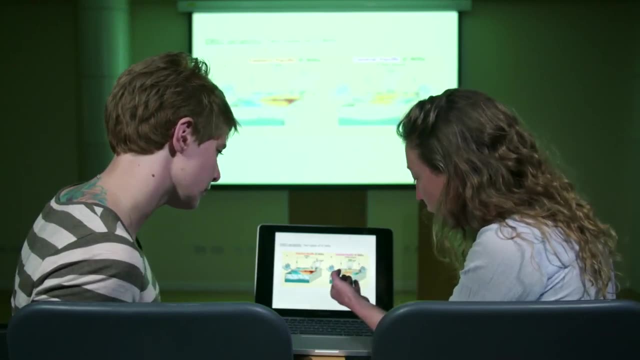 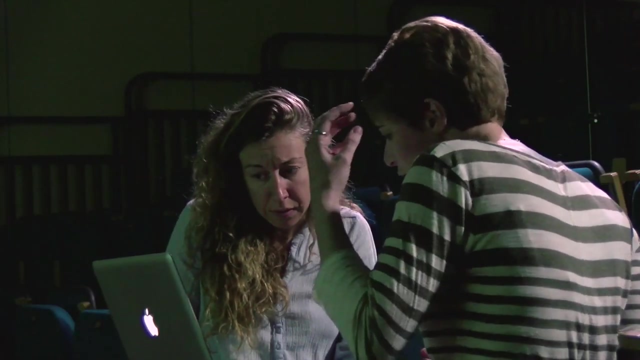 been an increased number of what they call the central pacific, El Niño, where the anomalous warming of SST- the maximum anomalous warming of SST- occur in the central tropical pacific. Okay, so we've got these two different types of El Niño, and this is all related to how the ocean 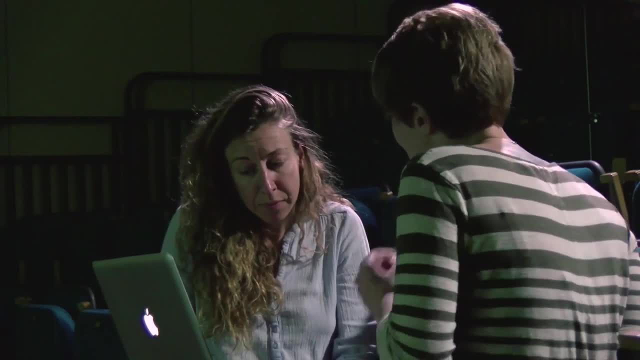 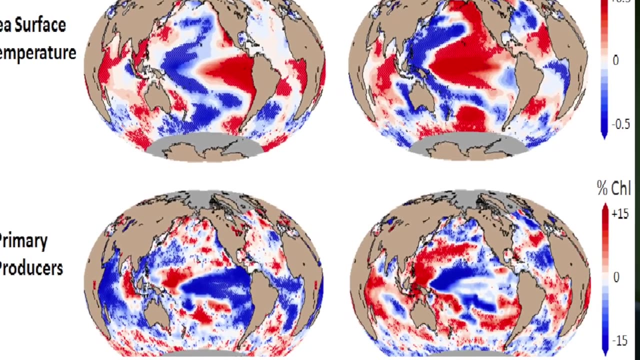 physics works and how the atmospheric physics works. but you said you've been studying the biology. so how does this connect to the biology? To study how it connects to the biology, basically we use some climate indices of El Niño variability to know when we have an eastern pacific, El Niño. 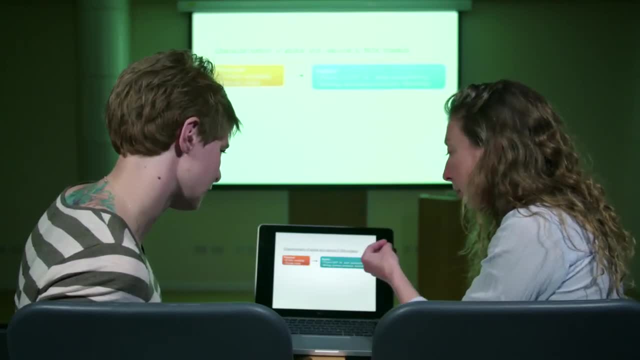 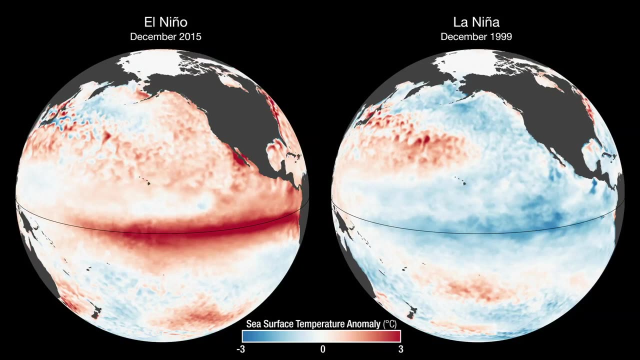 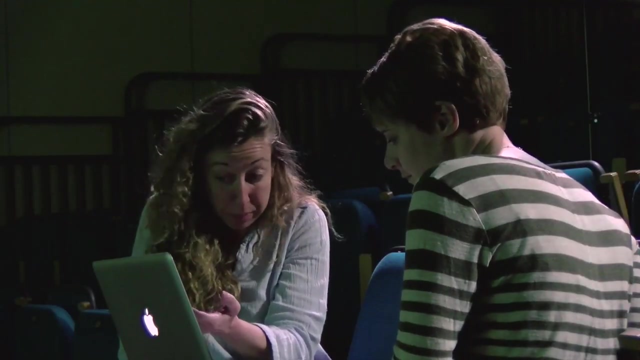 or a central pacific, El Niño, And we study the impact. so the impact on the physics. different physical variables are important for the phytoplankton to study the phytoplankton response, So mostly sea surface temperature, how it changes, changes in sea level, changes in wind patterns and wind direction. 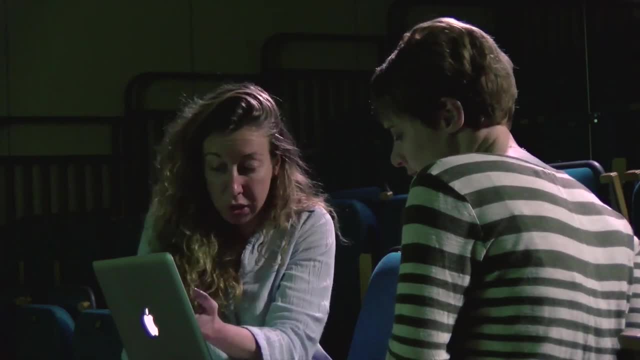 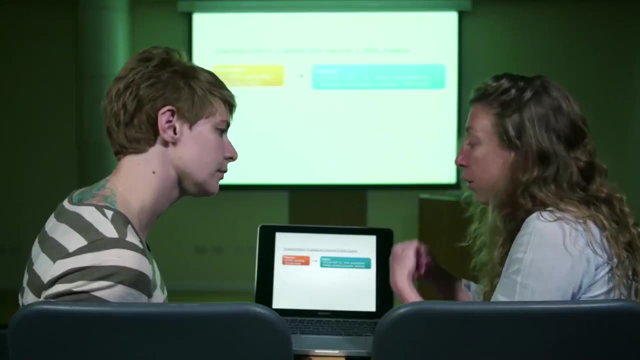 its strength and changes in precipitation, which might change the input from the rivers. The wind might change the mixing of the water column. it might bring nutrients to the surface which would allow phytoplankton to grow, So this is why it's very important. It might also change.